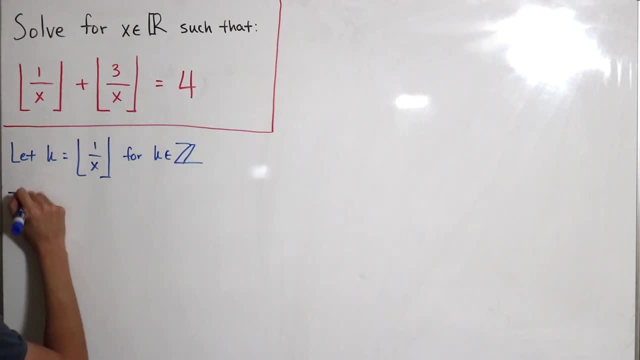 Then by using that definition, then that would have to say that k is less than or equal to 1 over x, strictly less than k plus 1.. But we also have one that's dealing with 3 over x as well for the floor function. 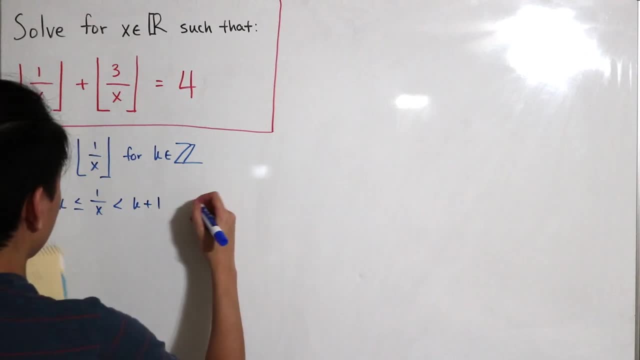 So let's actually put that to the side as well. So I'll denote this as a dash. that's saying that we have another one that we need to satisfy. So we just multiply 3 to the following over here. So then that will have to mean we have that 3 times k is less than or equal to 3 divided by k. 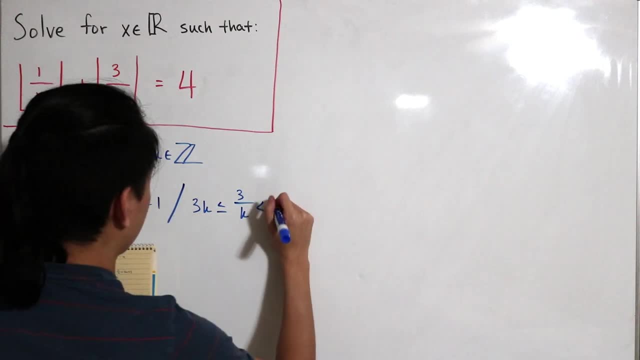 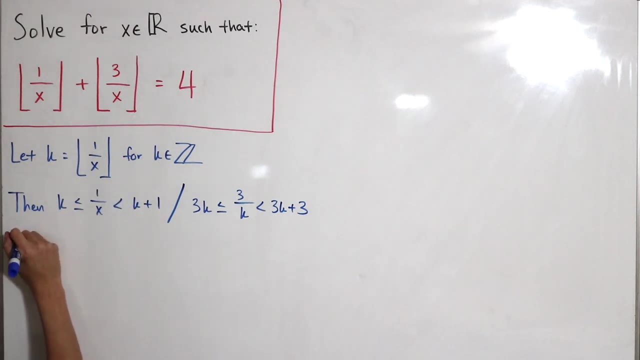 strictly less than 3 times k plus 1 or 3k plus 3.. All right, So now we actually just put in the substitution back so we know that we would have k. Then add this with the floor of 3 divided by x. 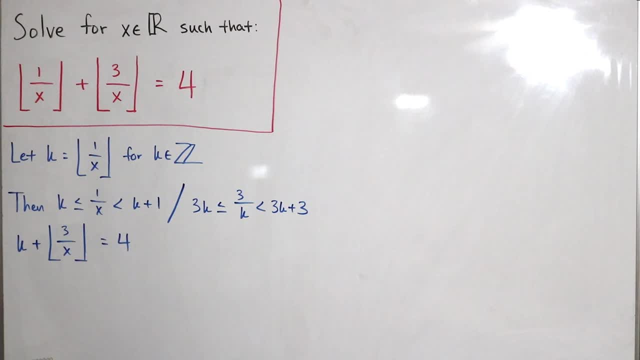 And then that's of course equal to 4.. But if we actually just said 3 over x- the floor of that by itself- then in other words we would have that This is just 4 subtract k. So let me just reiterate that. 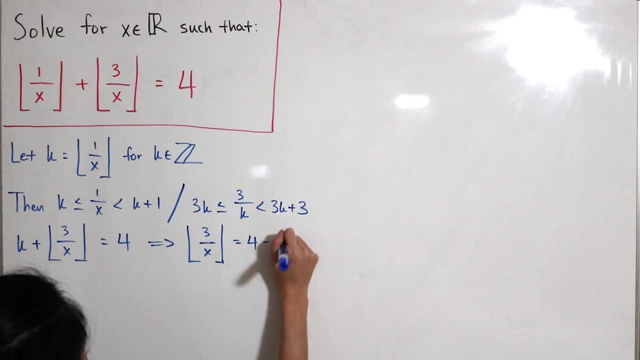 This equal to this will be 4 subtract k, So using this we can actually form ourselves a little inequality over here, So we can say that the inequality. so let me switch this back to pink. So we have the following inequality over here: 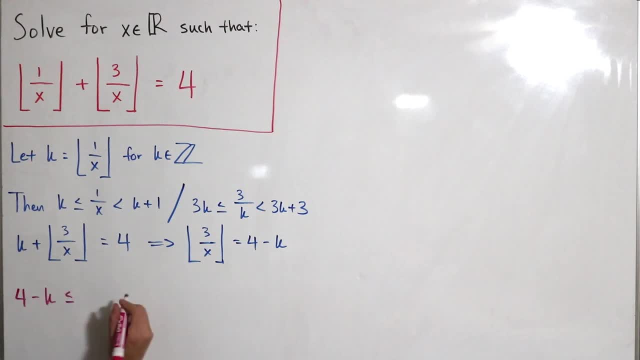 So we have that. this will be: 4 minus k is less than, or equal to 3 over x, which is less than, So add this by 1.. So this will be 5 subtract k. So now, with this inequality over here, we're actually going to analyze the following. 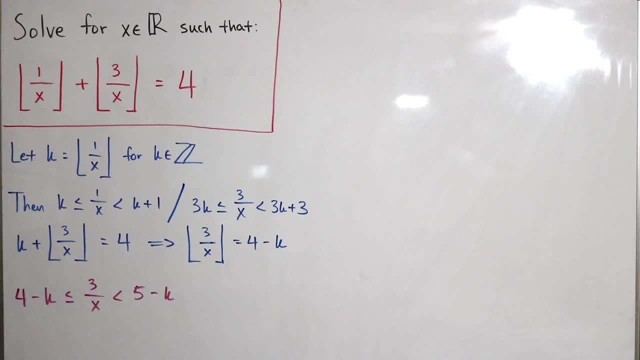 So we have: 4 minus k is less than or equal to 3 over x, And then 3 over x is strictly less than 3k plus 3.. So we'll actually just use that and analyze the following with 3 over x. 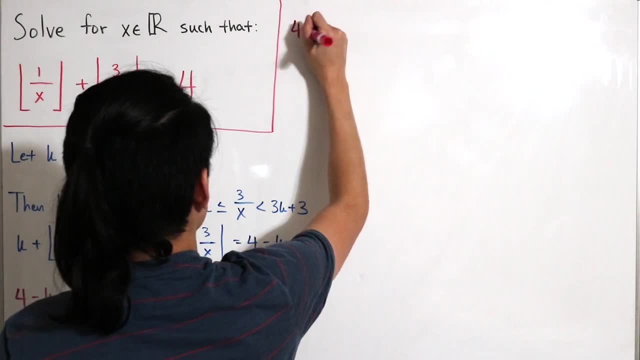 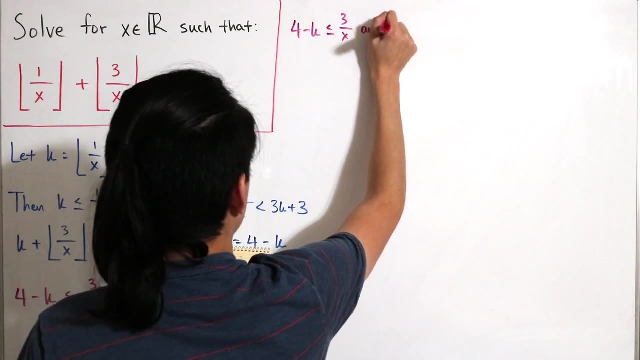 So in this case? so let's analyze 4, subtract k, which we said that that's less than or equal to 3 over x. Then we also want to focus that 3 over x is less than strictly less than, Less than 3k plus 3.. 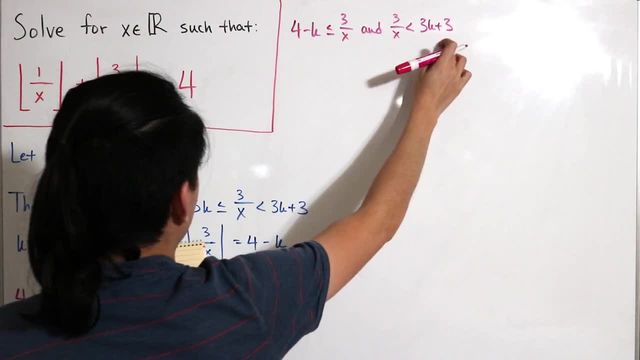 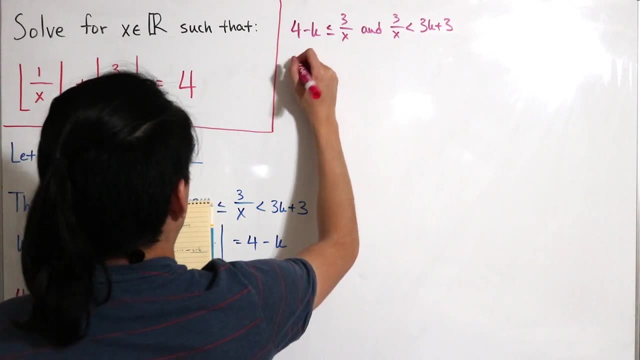 With this let's actually set the extreme left-hand side and right-hand side with the inequality, So with the comparison over there. So therefore we would say that we would look at: 4 minus k is strictly less than 3k plus 3.. 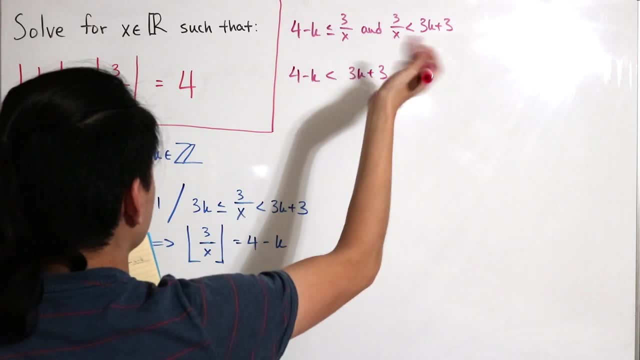 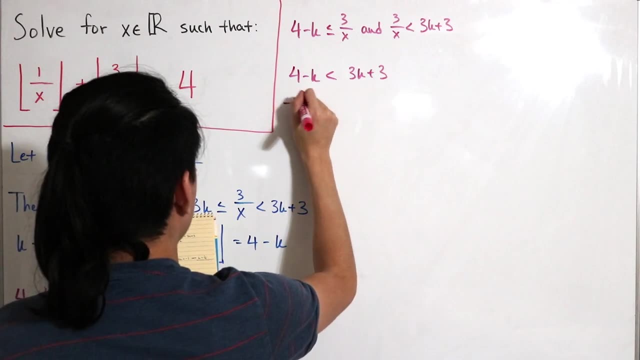 Okay, since they fall under the 3 over x, with that whole definition, with the integer or the floor function, So we just solve for k. That's actually pretty straightforward. We have 4, 4k, which is less than 1.. 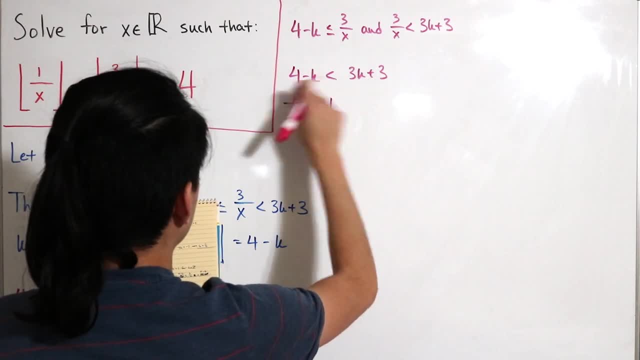 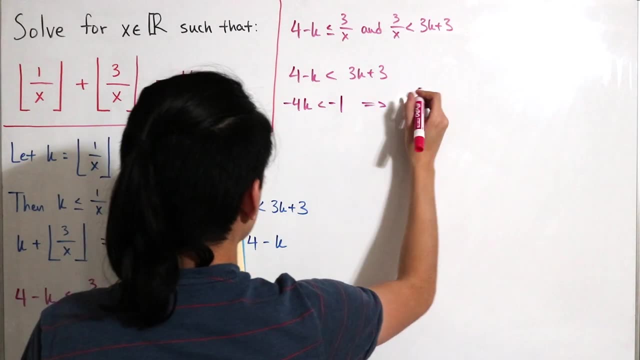 I just subtract the 3, then add the subtract the 3 to over here, then subtract the 4 over here. That's actually supposed to be a minus 1.. So negative 1.. Then we can see that this is just: k is well greater than or greater than 1 over 4.. 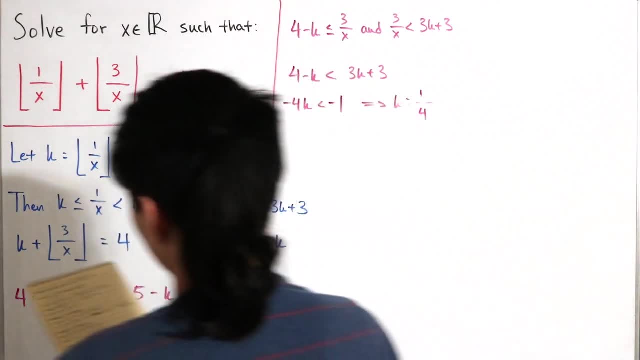 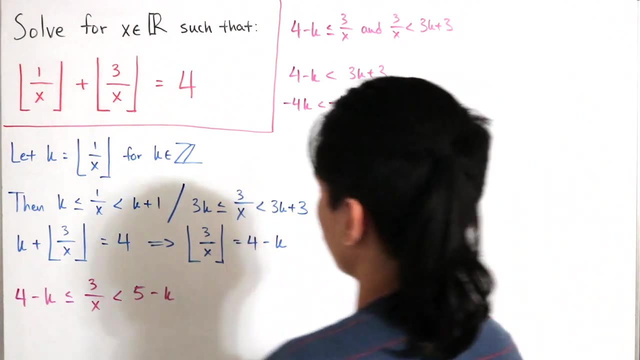 So we have one part of the inequality. So let's actually solve the other part which we have, that it's 3k is less than or equal to 3 over x. Then we also want to analyze the other part, with 3 over x is less than 5 minus k. 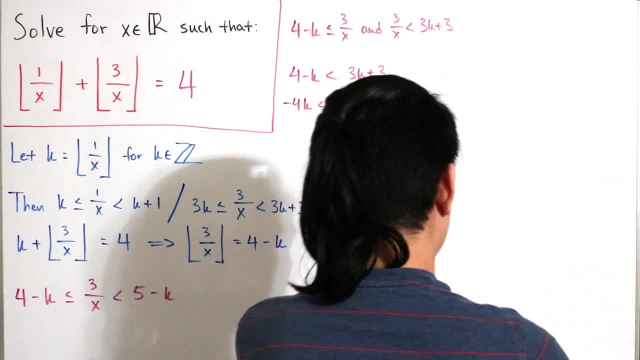 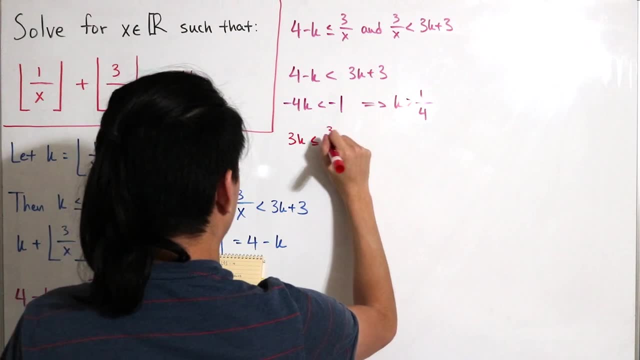 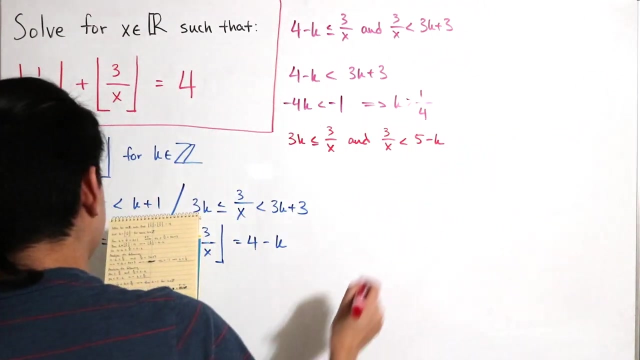 So let's pay attention to that and see what we can achieve from there. So we have 3k less than or equal to 3 over x and 3 over x less than 5 minus k. Apply that same technique, So 3k strictly less than 5 minus k. 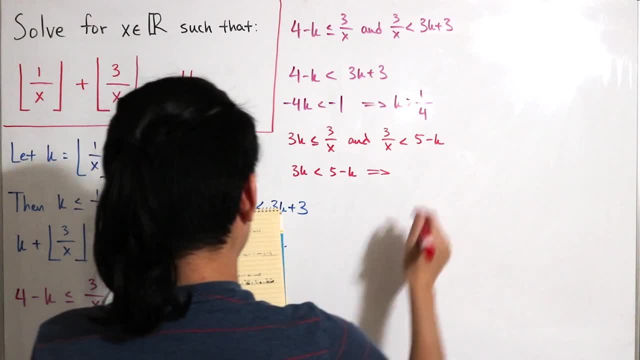 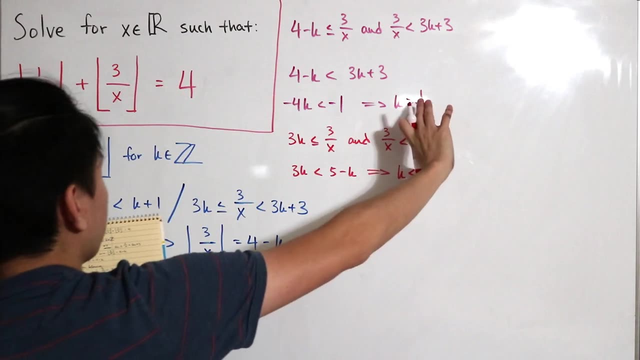 If we just solve for the inequality, Then we have that k is less than 5 over 4.. Okay, And if we just combine the inequalities together, everything is under 3 over over for under 3 over x. We're specifically looking at. 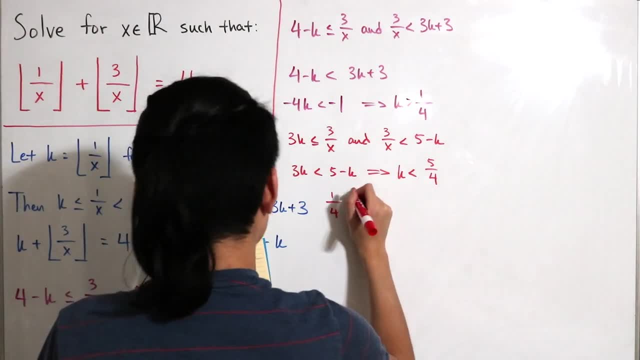 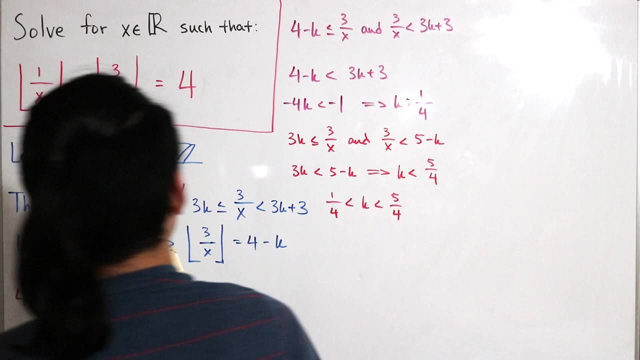 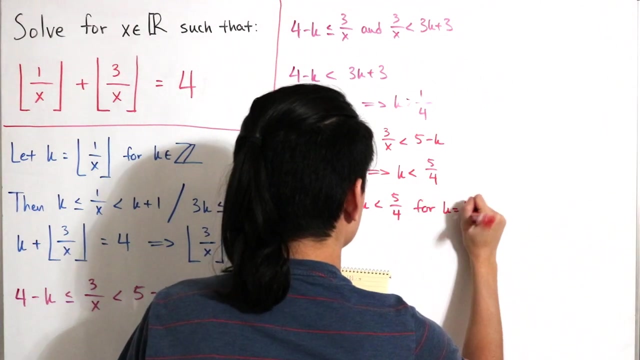 We formed the inequality that 1 over 4 is less than k, which is less than 5 over 4.. And notice that because we're looking at, k is for some integers. So in this inequality we see that This has to be, for k is equal to 1, for, you know, k is an integer. 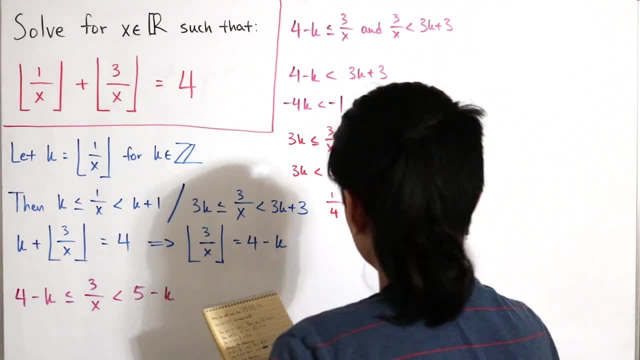 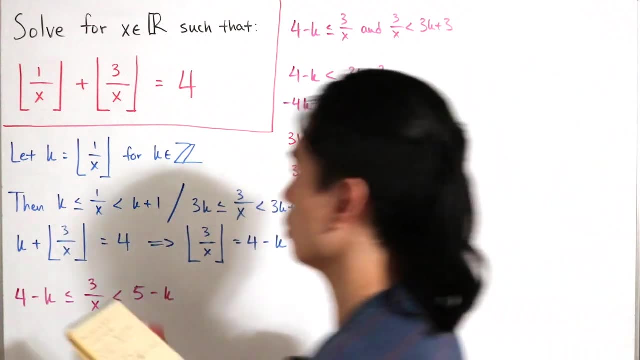 Okay, So now let's actually plug back. to plug k equals 1 back to our inequality. We're going to plug k equals 1 back to the this inequality over here. So let me just underline this: We're going to plug this back over here. 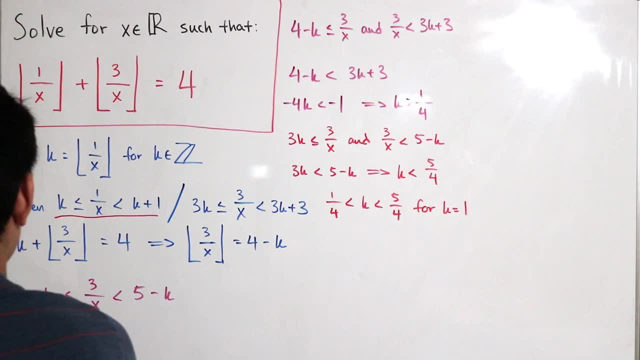 And then we're also going to plug the k equals 1 back to over here as well, Underline in red. So these are the two inequalities that we're going to plug. We're going to plug k equals 1 back in and see what we can get. 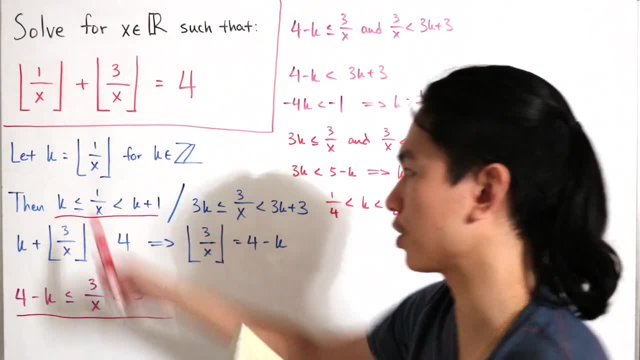 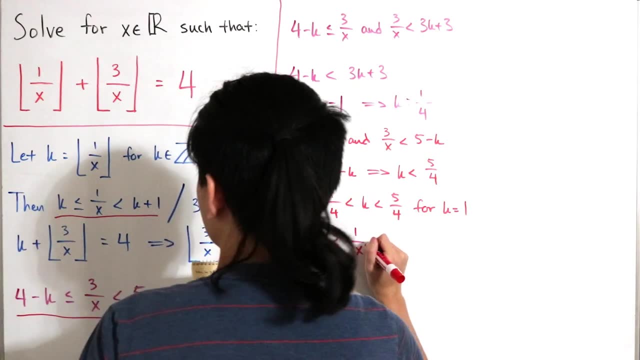 That means for. So if I plug, k equals 1 over here, so we'll just do this one step at a time. Then we have that this is just 1 less than or equal to 1 over x less than 2.. All right, 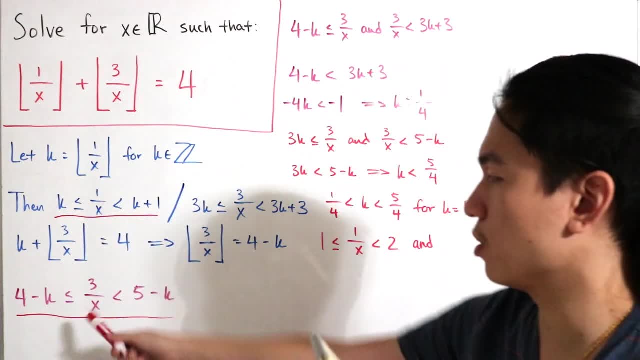 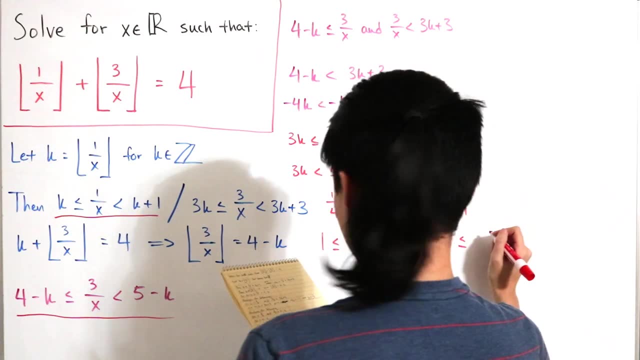 Then for the next part, I'll write an and Then, if we plug, k is equal 1. back to over here. So 4 minus 1, that is 3, which is less than or equal to 3 over x, Strictly less than 4.. 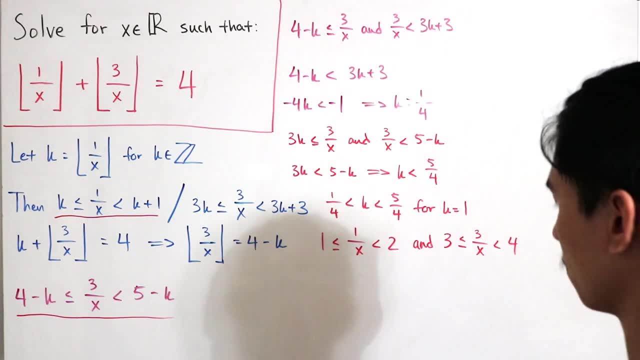 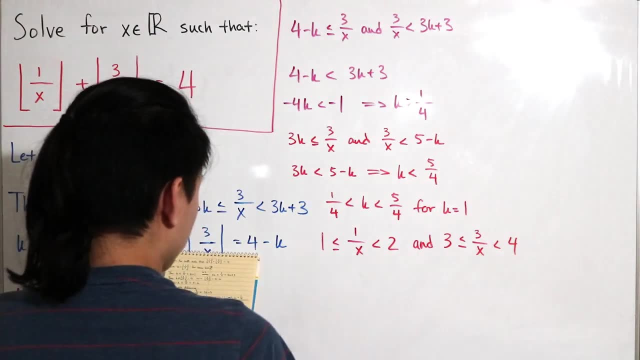 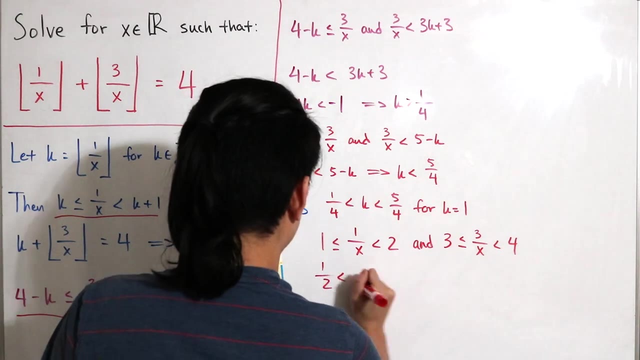 All right. So now let's actually just flip the reciprocal to both of these inequalities so that the center is just x. So that would also mean that we have to flip our signs as well. By doing so, we have that this is just 1 half strictly less than x, which is less than or equal to 1.. 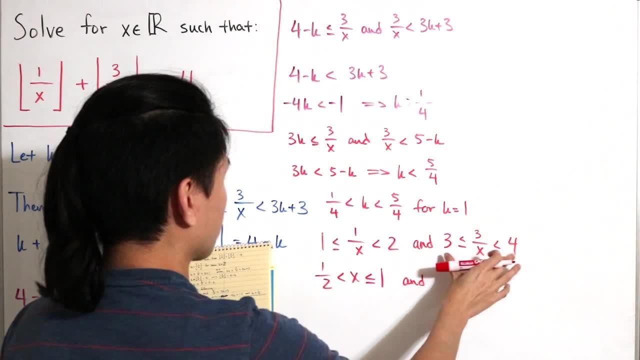 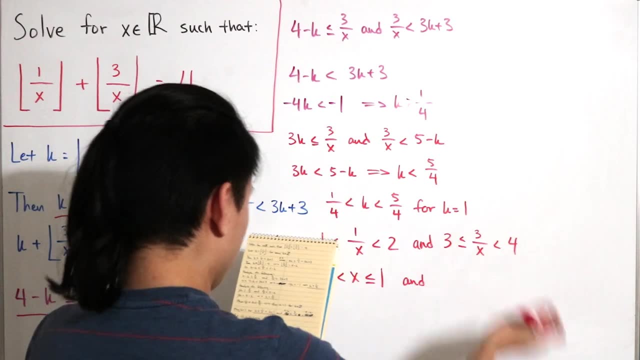 Then over here we flip the inequality or flip the reciprocal to everything. So this will just be 1 over 3.. This will be 1 over 4. But then you have to multiply 3.. And then, of course, the signs flip. 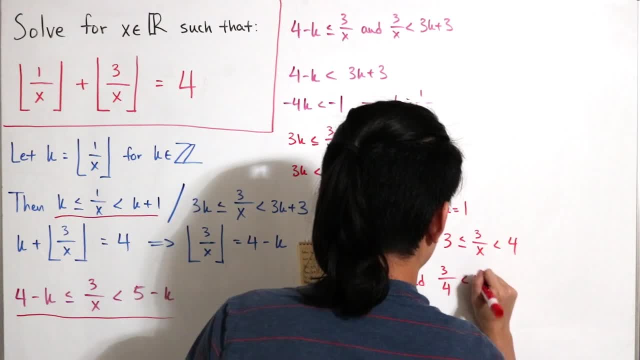 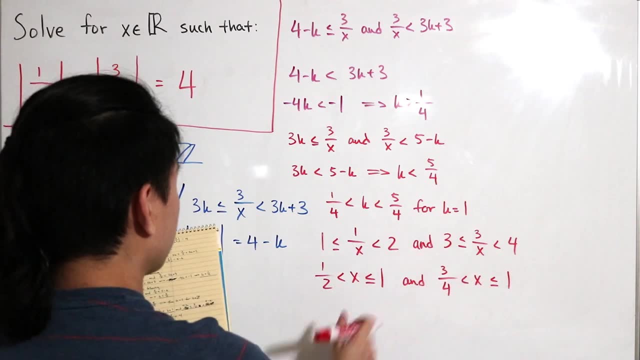 So that means we have that this is 3 over 4, strictly less than x, less than or equal to 1.. All right, And now from here is that if we just combine the inequalities together, we have of course 1 half is smaller than 3 over 4.. 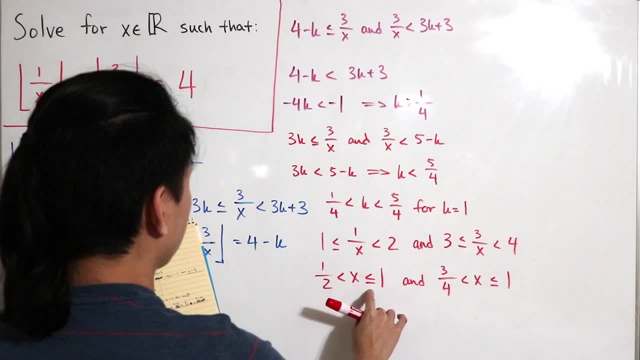 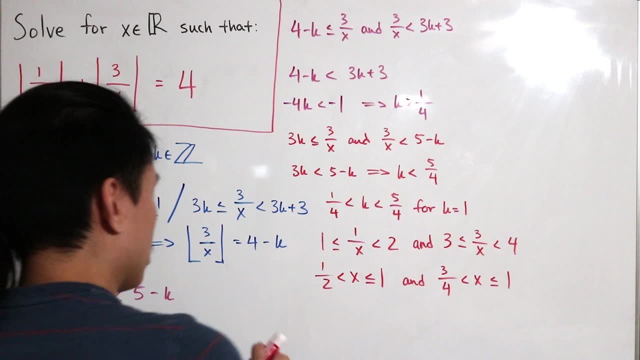 So we can just disregard this, because this is also with the greater, less than or equal to 1, just like over here. So we just pay attention to that. The only really thing is that x Can fall between 3 over 4 and 1 inclusive.